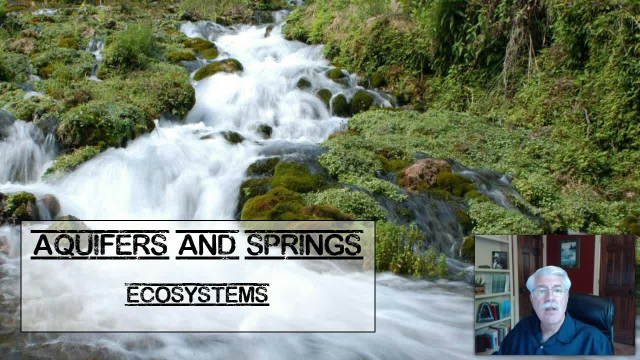 Now these can support entire ecosystems that include invertebrates, fish and amphibians, all deep under the ground, But these species are unlike anything we're used to seeing above ground. The aquifer has no sunlight and therefore no green plants or algae with chlorophyll that. 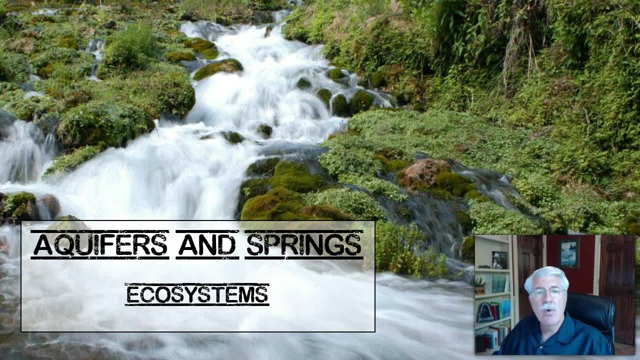 take the sun's energy and convert it to food. Without these primary producers, the aquatic ecosystems underground don't have a lot of nutrients or food, So they can't live in the crystal clear soils, especially when there's no natural resource Available. food is constantly recycled among the organisms that are there, with only occasional. 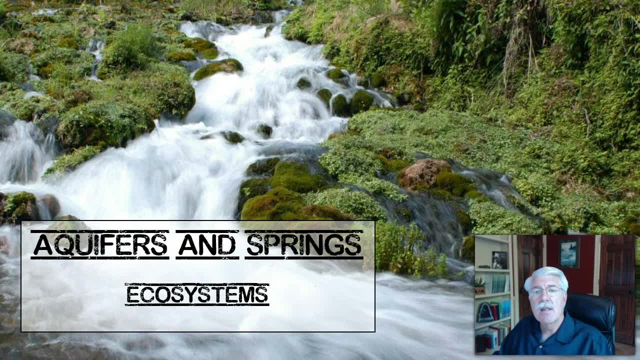 additions of food from the outside. These underground ecosystems have a very low carrying capacity. as a result, They can only support a few individuals of any one species, and these individuals usually don't grow to be very large at all. This lack of sunlight has another 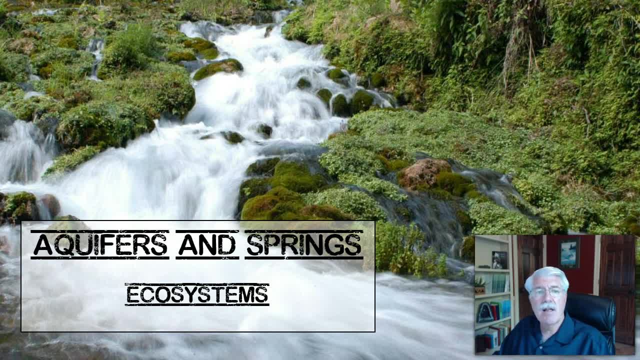 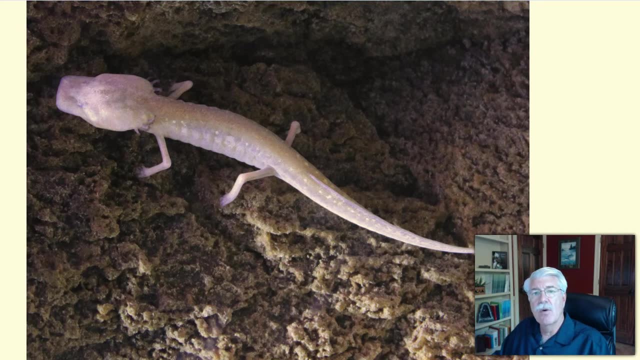 consequence. In fact, the single most amazing adaptation of invertebrates, fish and amphibians to the dark underground aquatic ecosystem is an absence of eyes. Here we see the Texas blind salamander. It's adapted for living in these water-filled caves of the Edwards Aquifer. 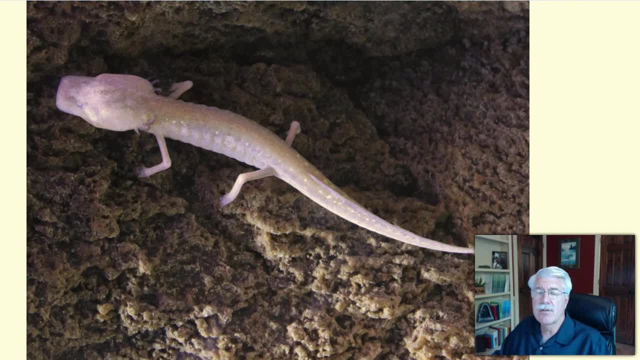 It has no eyes. It does have two small black dots under the skin where eyes would normally be. yet the blind salamander is an active predator. It hunts food by sensing water pressure waves that are created by prey in the underground waters where it lives. 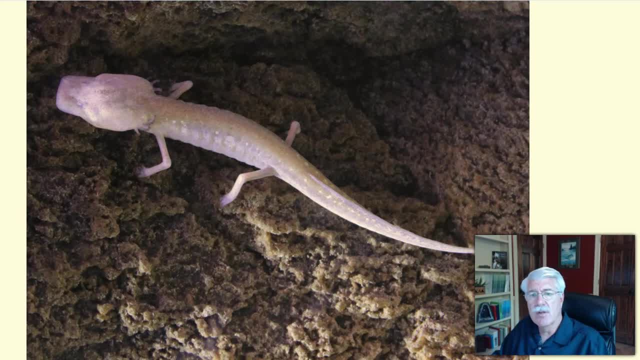 There are no waves or great currents there, so even the slightest movement of water can be detected by these little predators. Tiny snails, shrimp and other aquatic invertebrates make up its diet. It also has very little skin pigment. Its color is white and in some places, clear. 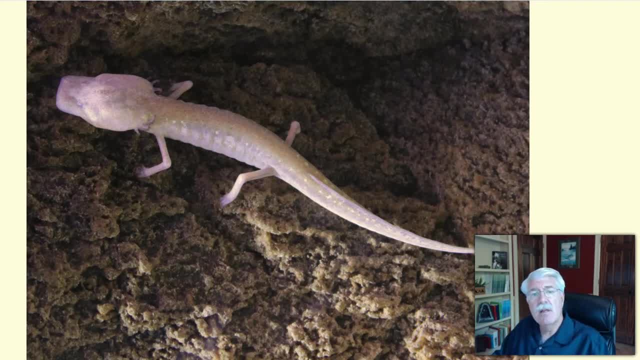 The skin is just clear right through and it has red external gills that are used to get dissolved oxygen from the water. It's unknown how many Texas blind salamanders really exist In these deep underground waters. predators have adapted ways to find and catch prey in. 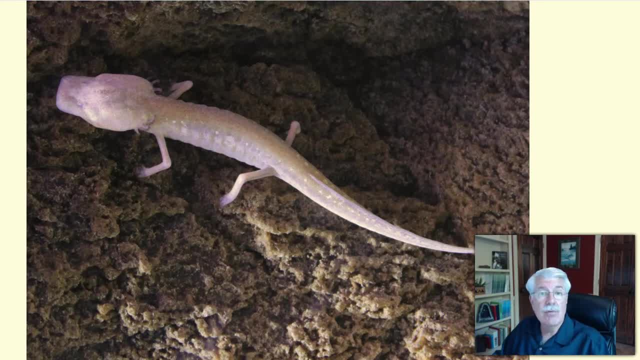 the dark And prey have adapted ways to escape. Sensory adaptations such as antenna chemoreceptors and touch receptors are highly developed in these underground dwelling species. These species also have a very low metabolism, allowing them to live on very little food. 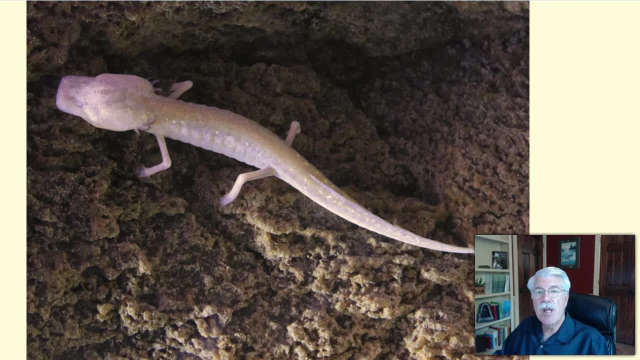 This adaptation is aided by the constant temperatures of aquifer waters. This is compared to surface water temperatures, which can vary very quickly and widely. This adaptation is aided by the constant temperatures of aquifer waters. This is compared to surface water temperatures, which can vary very quickly and widely. 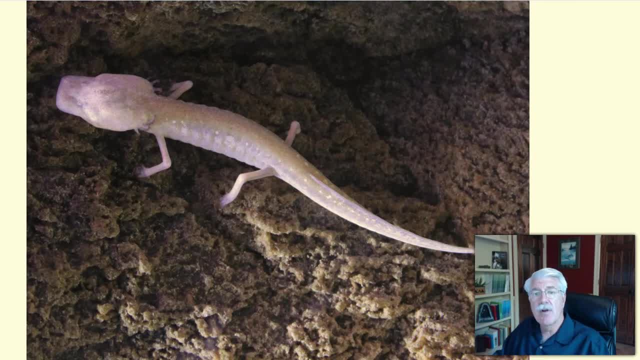 Groundwater species live in a very stable and predictable environment, As with aquatic ecosystems. above ground, though, there can be overlaps with other ecosystems. This means that species in the aquifer may not be completely isolated from life on the surface. The land surface above the karst aquifer is an integral part of the habitat of animals. 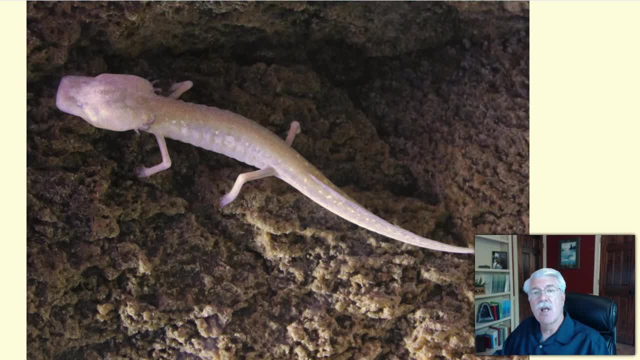 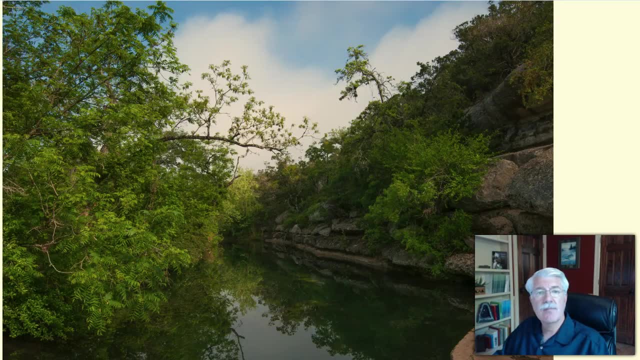 that inhabit the underground areas. Holes in the limestone and marble of these aquifers often extend to the surface. Holes in the limestone and marble of these aquifers often extend to the surface. Holes in the limestone and marble of these aquifers often extend to the surface. 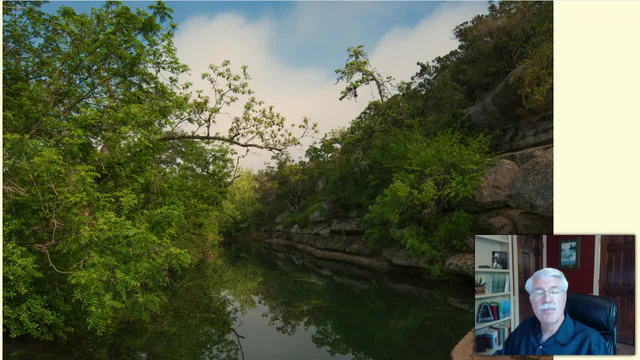 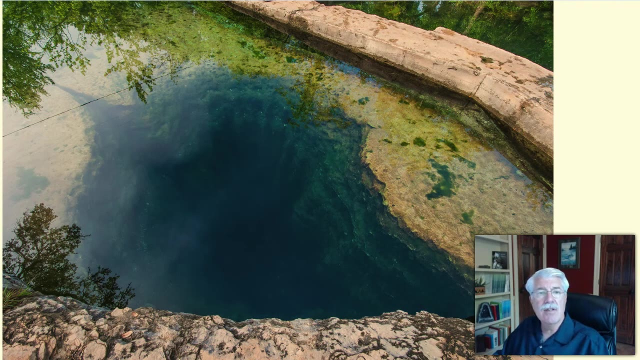 Jacob's Well near Wimberley is a good example. Here is a large opening in the streambed of Cypress Creek. This opening is actually a water-filled cave that extends deep down into the aquifer. Here is a large opening in the streambed of Cypress Creek. 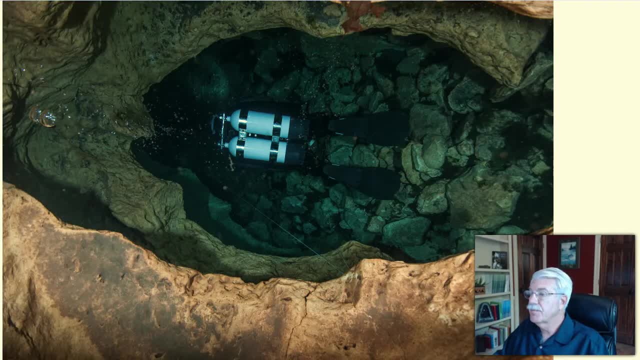 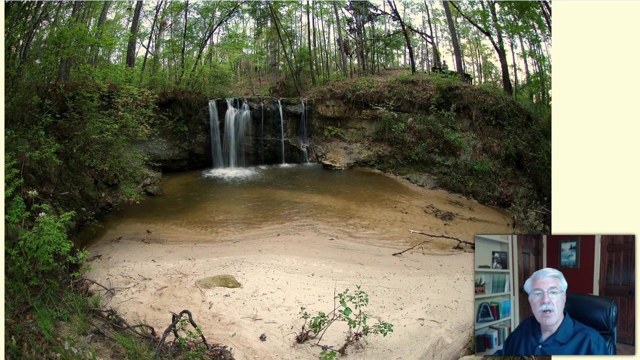 that lead to the aquifer and many other locations. Because plants can't grow in darkness, the cave and associated underwater ecosystem is dependent on plant and animal materials being washed into the cave from the outside. Food in the cave can also come from organisms such as bats, mice and crickets that take shelter in caves. 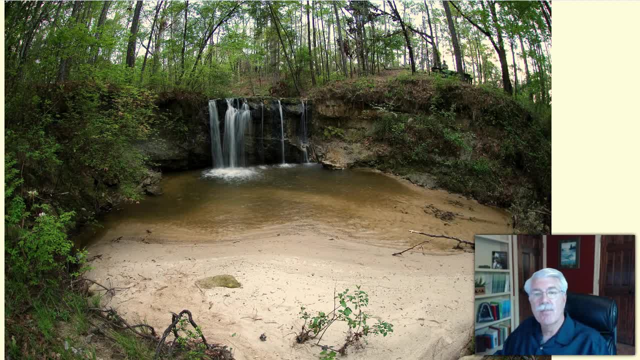 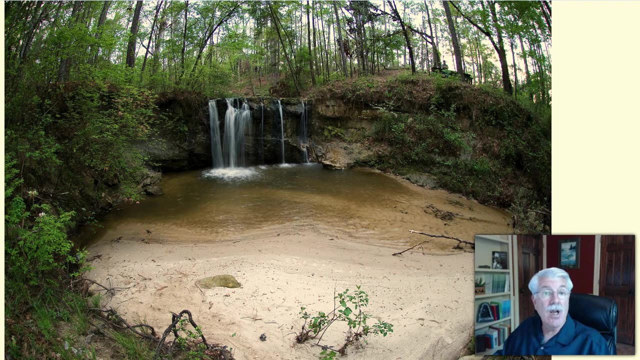 They can become food or prey for cave dwellers, or they can also leave food behind. For example, bat and mouse feces dropped on a cave floor provides nutrients that fungi need to grow. Fungi are eaten by several species of insects that may wander in and out of the cave. 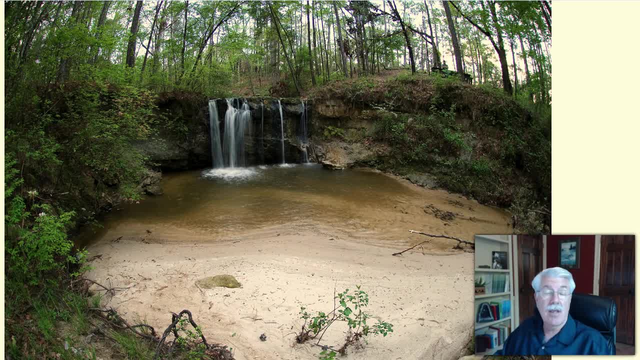 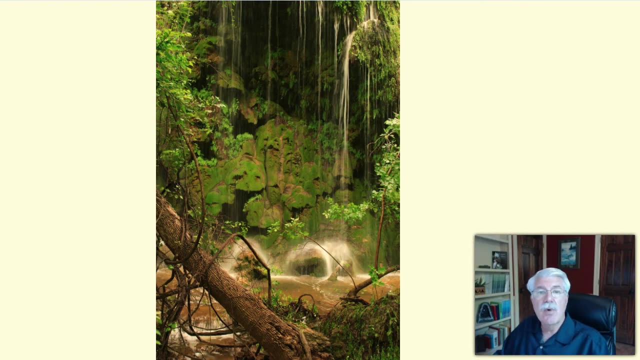 These insects produce very rapidly, they move about the cave and they become prey for predatory invertebrates that live their entire lives in the cave. These invertebrates fall into the water and can be swept deep into the aquifer, where they can be eaten by species. 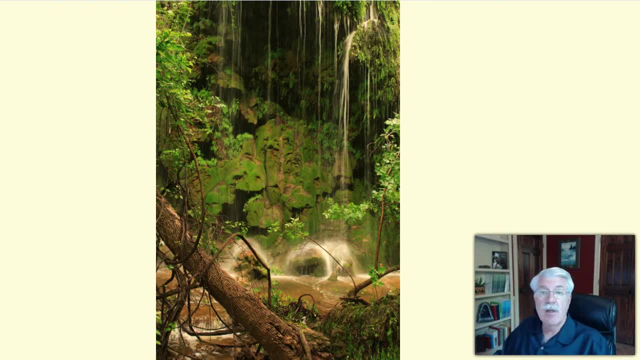 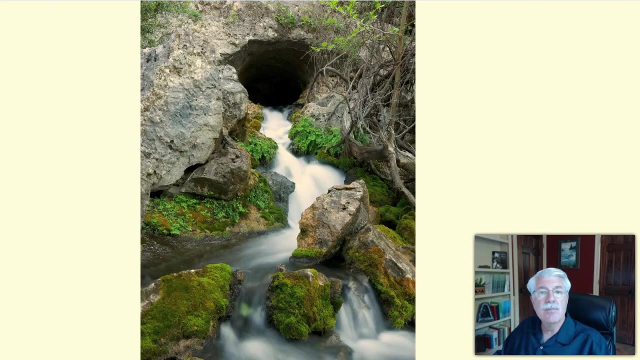 such as the Texas blind salamander. Now the salamander itself can be eaten by other species, such as the toothless blind cat. This is a catfish that can live over 1,000 feet below the Earth's surface. The aquifer ecosystem extends beyond the aquifer itself. 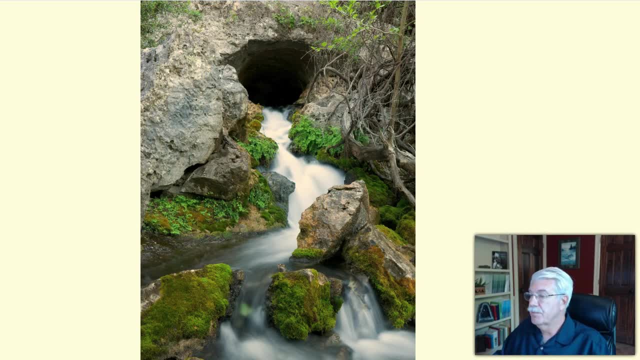 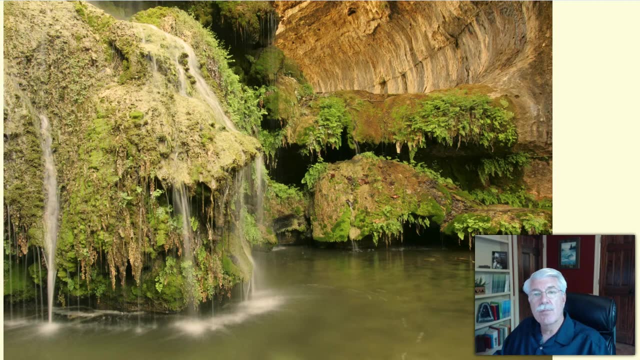 where groundwater emerges into a spring. Here, the groundwater mixes with surface water in the spring stream, rivers, and lake water is downstream. However, it is not a water source. It is a water source. It is in the springs themselves that are formed by the aquifer's emerging waters. 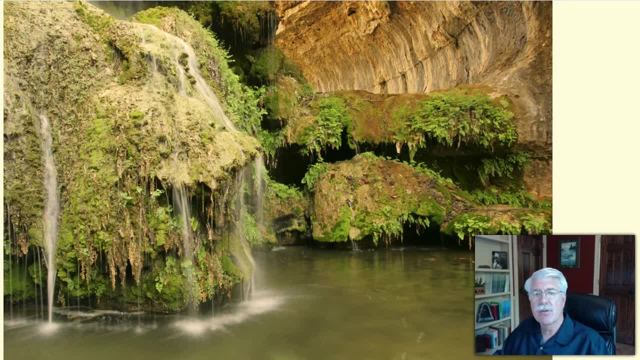 where the unique underground ecosystem truly extends to the surface. We occasionally get a rare glimpse of life in these underground ecosystems. when an invertebrate fish or salamander from the Edwards Aquifer, for example, gets swept out into a spring, You may see one of these odd creatures. 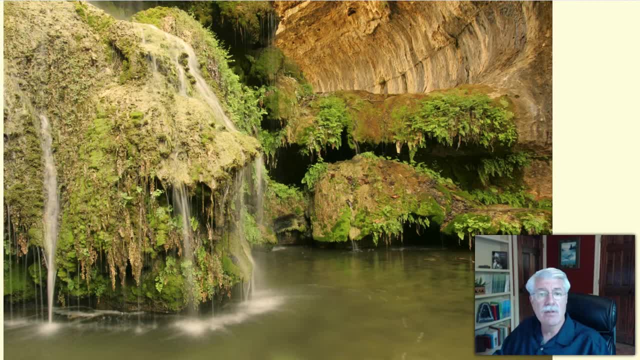 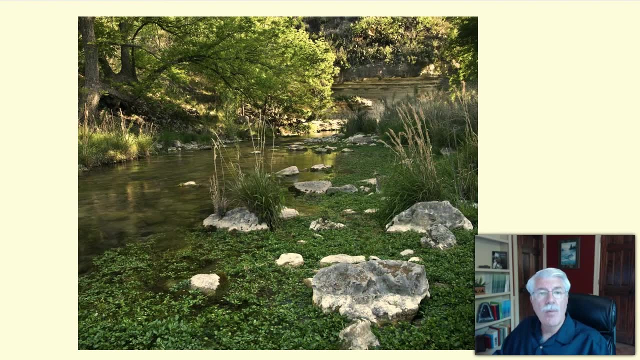 or one of the predators that like to eat them when you tour the San Marcos Springs in a glass-bottomed boat. While many aquifers don't contain aquatic life, most major springs in Texas do. Some even contain species found nowhere else: The Edwards Aquifer ecosystem and its springs. 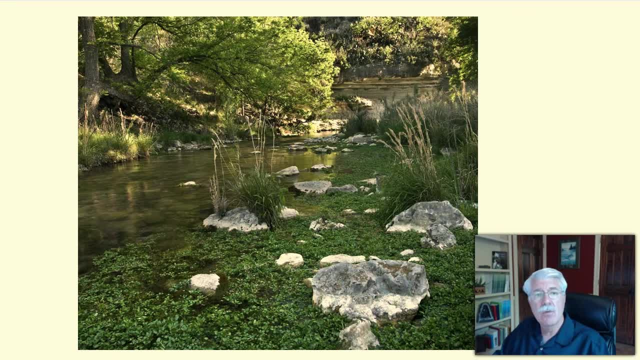 contain over 60 species of plants and animals that live nowhere else in the world. Species of salamanders, fish, amphipods, beetles, spiders and others have evolved in these isolated habitats within the aquifer and spring. Many of these live in the dry caves above the water table. 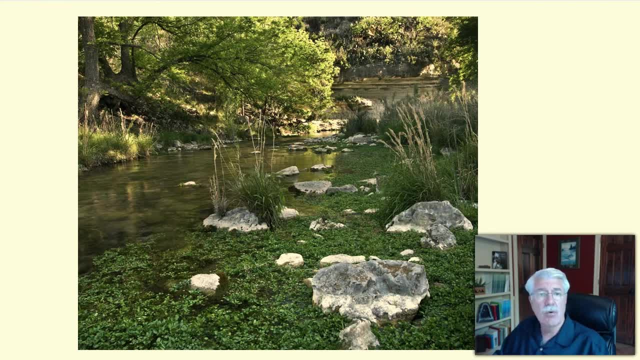 and others live in the many springs fed by the aquifer. Barton Springs, located in Austin, is the only place where the Barton Springs and Austin blind salamanders live. Fountain darters live only in the San Marcos and Comal rivers. Texas wild rice lives only in the San Marcos Springs.